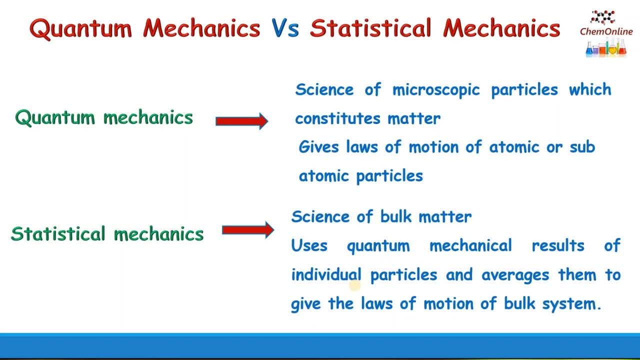 Now let us see what is the difference between quantum mechanics and statistical mechanics. Quantum mechanics is a science of microscopic particles. Quantum mechanics is the science of microscopic particles and gives the laws of motion of atomic or subatomic particles At the same time. statistical mechanics is a science of bulk matter and it 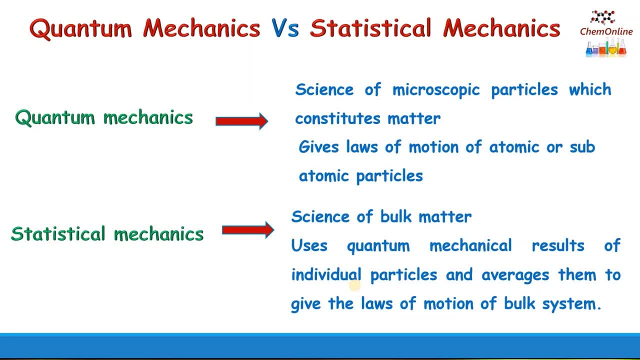 uses quantum mechanical results of individual particles. In quantum mechanics, we do not consider the particle as a whole or the system as a whole. We deal with each and every atom or subatomic particles. So we deal with each and every atom or subatomic particles. So we deal with each and every. 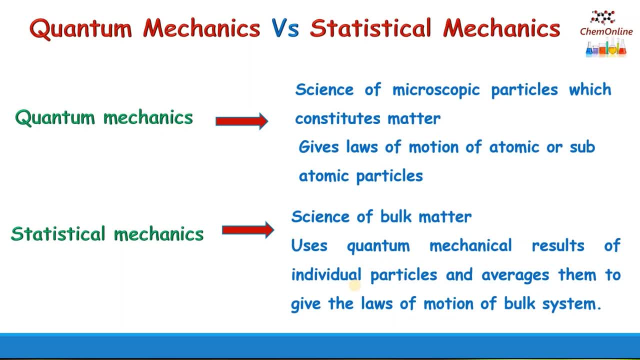 atom or subatomic particles. So we have to evaluate the microscopic properties of the particles, For instance the nuclear distance, the moment of inertia, etc. so we evaluate them quantum mechanically and then we apply them to the system as a whole. We then average. 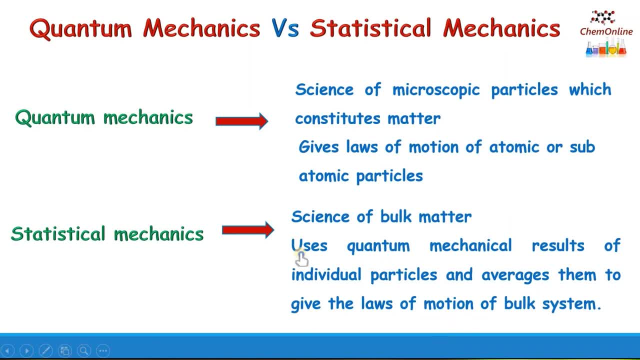 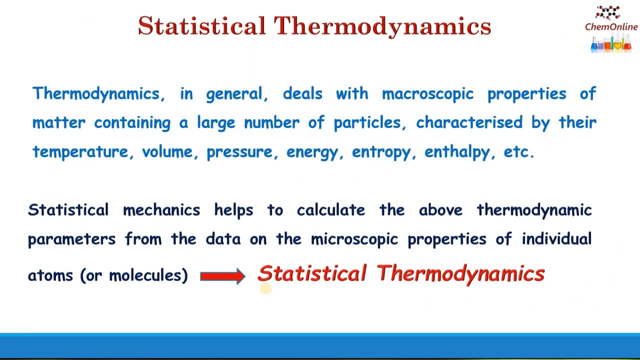 the loss of motion of the bulk system. This is the main difference between quantum mechanics and statistical mechanics. What is statistical thermodynamics, Thermodynamics, Thermodynamics- In thermodynamics we deal with macroscopic properties of the matter. The large number of particles, particle as a whole, system as a whole, are what we consider. 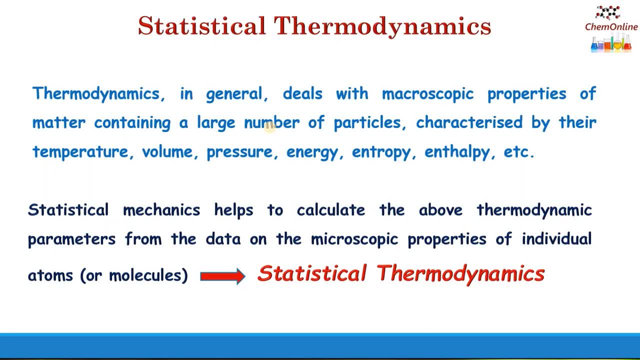 And they are characterized by the temperature, volume, pressure, energy, entropy. These are all macroscopic properties. They characterize the system as a whole. These are the properties that characterize the system as a whole. That is what we deal with in thermodynamics. 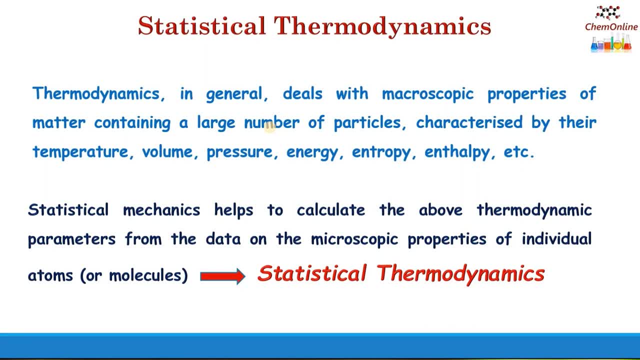 In statistical mechanics. it helps to calculate these thermodynamic properties, like volume, pressure, energy, etc. from the data on the macroscopic properties of individual atoms or molecules using laws of statistical mechanics. That is why it is called statistical thermodynamics, Because we finally evaluate the thermodynamic properties. 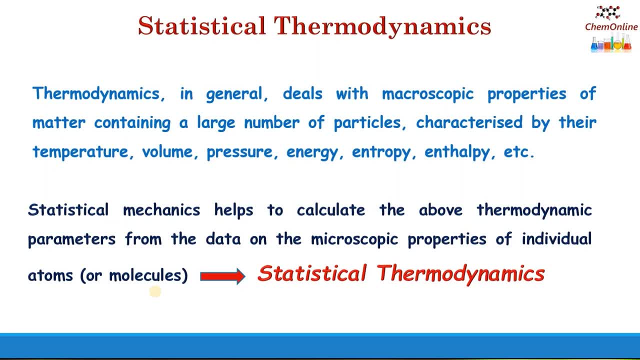 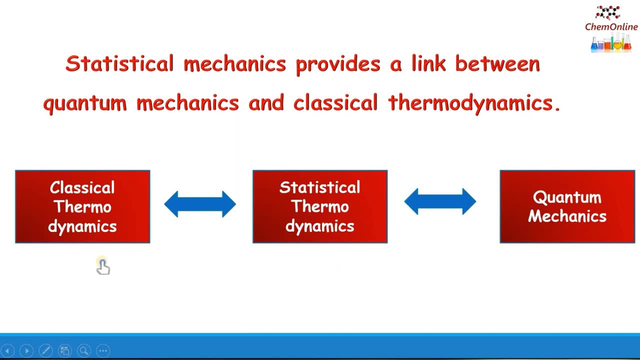 Hence statistical mechanics is also known as statistical thermodynamics. Statistical thermodynamics is a bridge between quantum mechanics and classical thermodynamics. These two branch names connect in a link. Classical thermodynamics name and quantum mechanics name connect in a link in statistical thermodynamics. 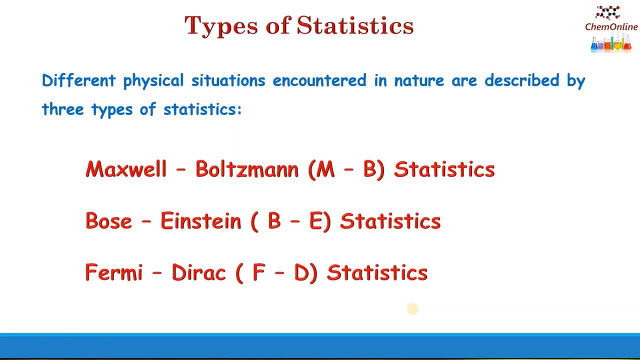 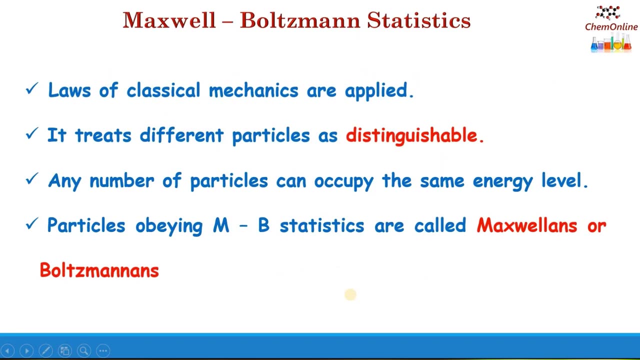 Now we have different types of statistics: Maxwell-Boltzmann statistics or MB statistics, Bose-Einstein statistics, abbreviated as BE statistics, And Fermi-Dirac statistics, And Maxwell-Boltzmann statistics, abbreviated as FD statistics. So what is Maxwell-Boltzmann statistics? 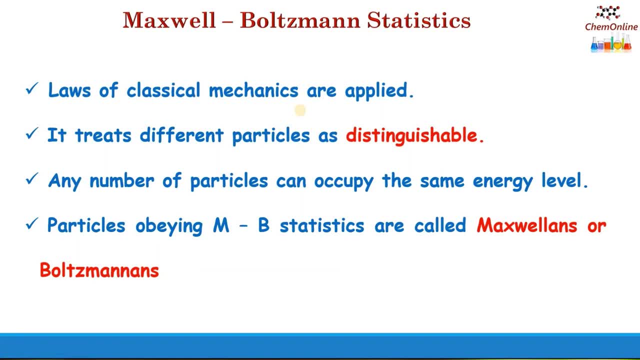 Laws of classical mechanics are applied. Classical mechanics means we apply Newton's laws of motion. You must have studied in elementary class First law, second law, third law, etc. Classical mechanics is a branch of Newton's laws of motion. Maxwell-Boltzmann statistics follows classical mechanics. 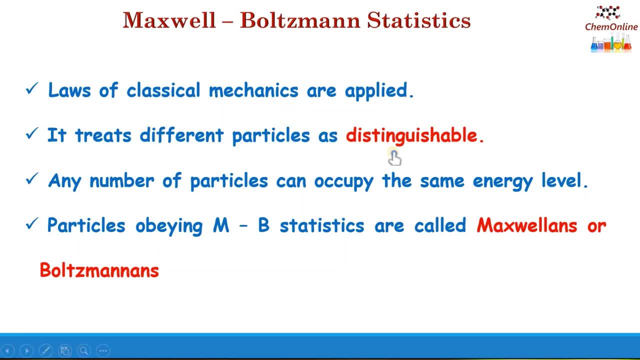 It treats different types of statistics. It treats different particles as distinguishable. It treats particles as distinguishable. We can know that it is treatin distinguishable Now. any number of particles can occupy the same energy level. It can occupy the same energy level at any number of particles. 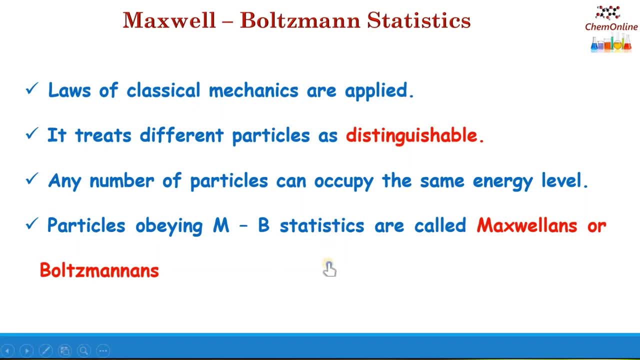 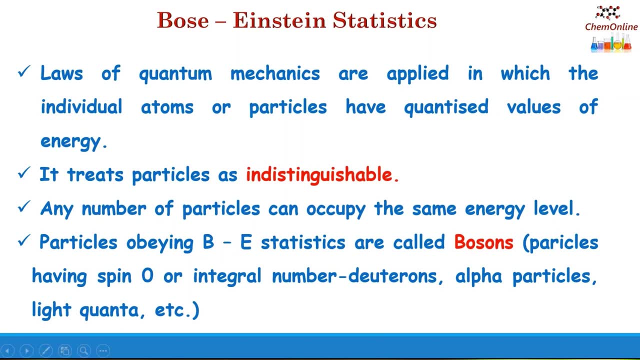 And particles obeying MB statistics are called Maxwell-Boltzmann or Maxwell-Boltzmann. Now next is Bose-Einstein statistics. In Bose-Einstein statistics, laws of quantum mechanics are applied. Quantum mechanics, individual atoms or particles have quantized values of 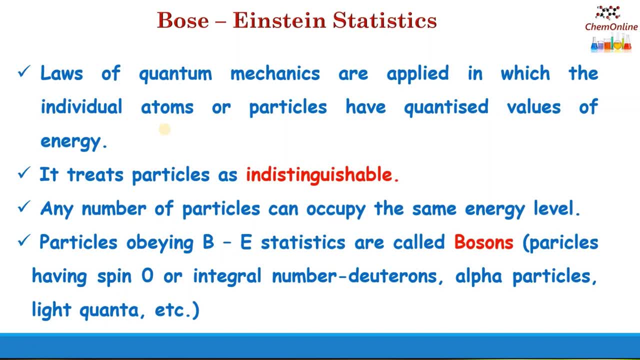 energy, Whereas according to classical mechanics the particles have any value of energy. But here laws of quantum mechanics are applied, in which the atoms or particles have quantized values of energy. It treats particles as indistinguishable. Any number of particles can occupy the same energy level. 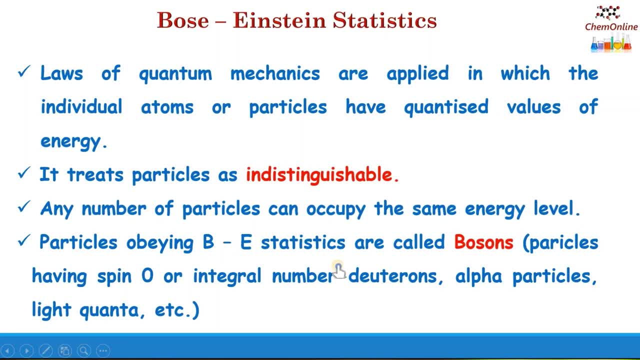 And particles obeying these statistics are called bosons, Particles having spin 0 or integral number or all obey Bose-Einstein statistics. So example here is deutrons, alpha particles. Alpha particles are helium, nuclei, 2He4.. Light quanta, etc. all obey Bose-Einstein statistics. 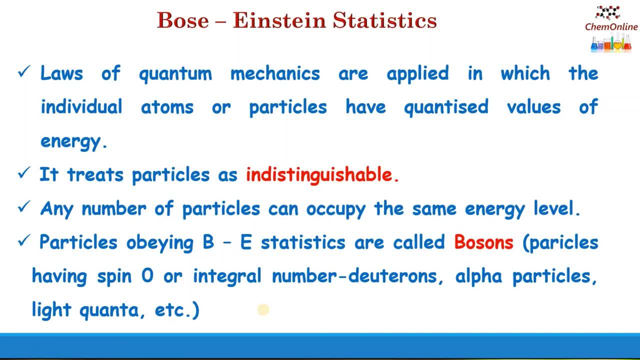 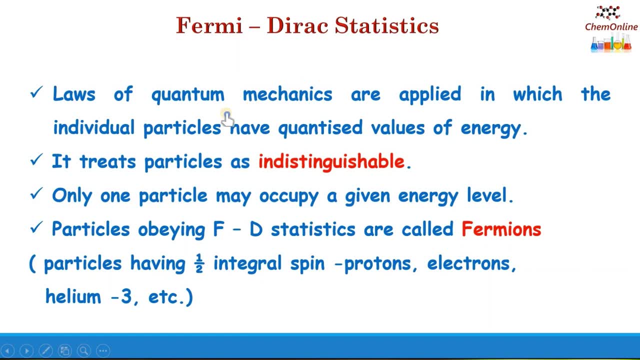 And particles obeying such statistics are called bosons, And the next is Fermi- Dirac statistics. Laws of quantum mechanics are applied here also. It follows the laws of quantum mechanics. It treats particles as indistinguishable. Now there is a difference from the other. 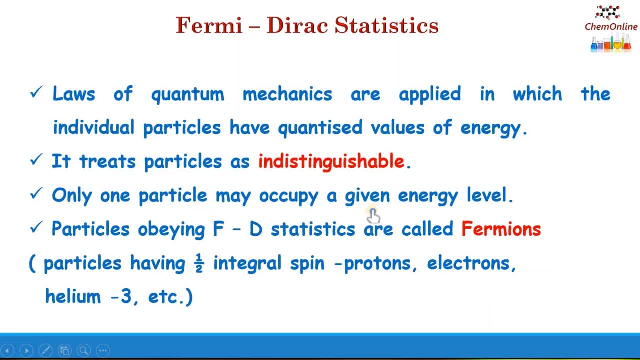 two statistics: Here only one particle can occupy a given energy level. A restriction arises here. Here one particle can occupy a given energy level. A restriction arises here: Here one particle can occupy a given energy level. here There is a restriction that there is only one particle that can occupy a inertia level. 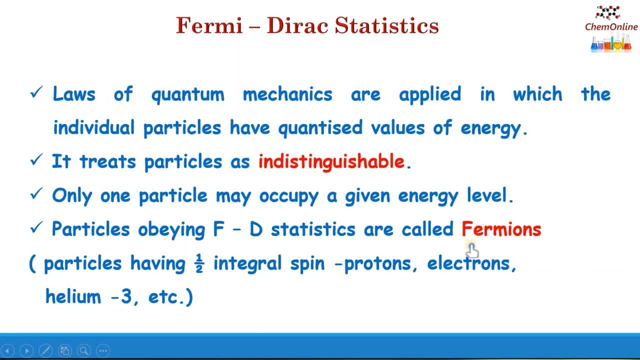 Now, particles obeying FD statistics are called fermions. A very good example for a fermion is electron. All particles having half integral spin are fermions, For example protons, electrons, helium-3, etc. So these are the three different types of statistics and we have seen 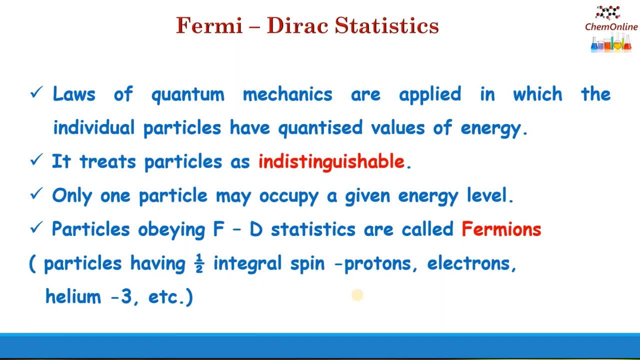 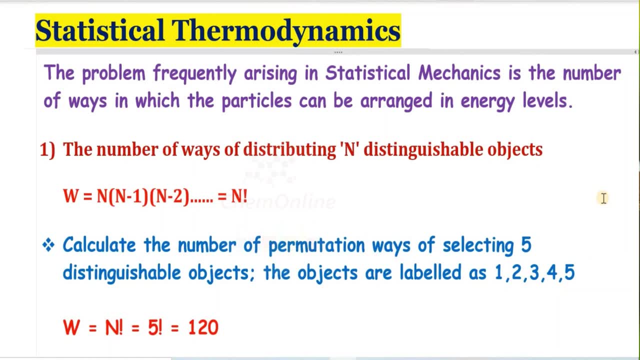 brief properties of different types of statistics. We usually deal with a problem in statistical mechanics: how to arrange particles at different energy levels. So the problem frequently arising in statistical mechanics is the number of ways in which the particles can be arranged in energy levels. So you can see the first case. 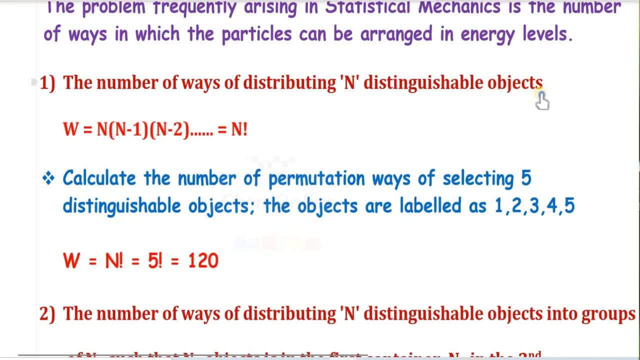 the number of ways of distributing N distinguishable objects. If you have N distinguishable objects, then they can be arranged in N, into N minus 1, into N minus 2, into N minus 3, etc. So this is equal to N factorial. 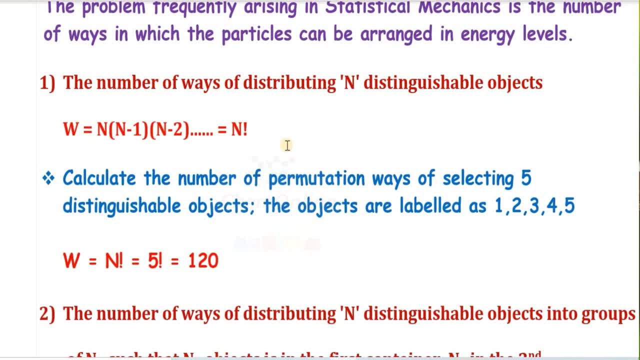 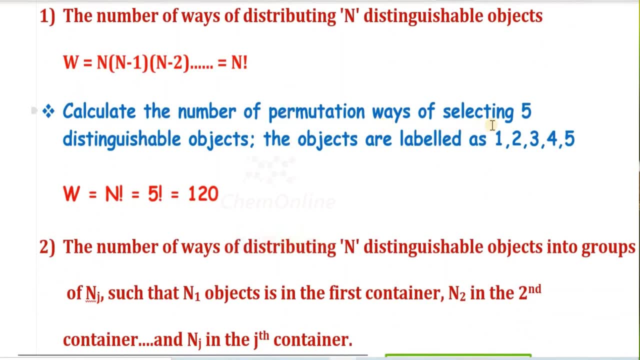 Again N distinguishable objects. and again you can arrange it in N factorial ways. I have given an example here. Calculate the number of permutation ways of selecting five distinguishable objects. The objects are labeled as 1,, 2,, 3,, 4,, 5, etc. So you have five distinguishable objects. So in how many ways you can arrange. 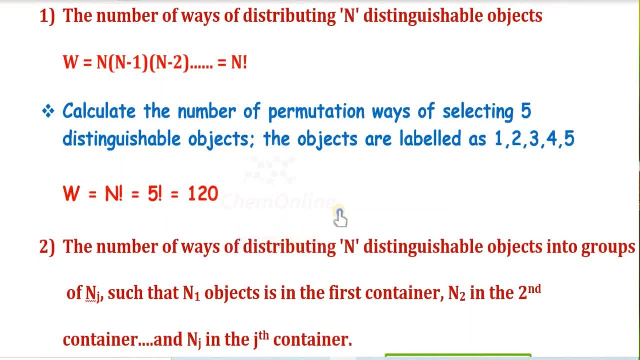 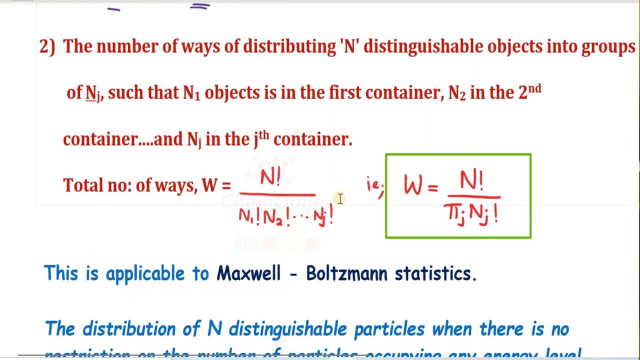 five distinguishable objects. So according to the equation, W equals N factorial. So if N is 5, 5 factorial, which is equal to 120.. Now next is number of ways of distributing N distinguishable objects into groups. 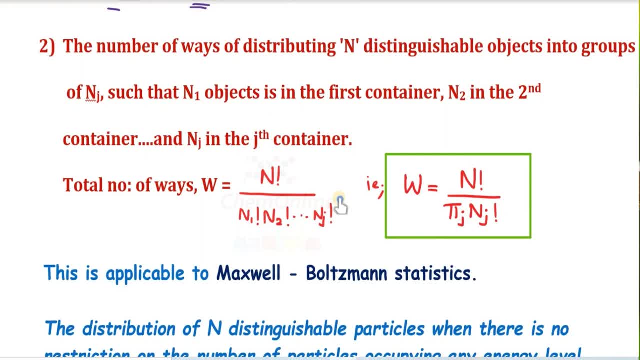 N0.. N rules that we have enough to write 2, N and items in Gまり. Now C has to determine M irgendwie. Once you have this four distinguishable objects, you can say that the RN in first container is equal to green, from 0 to yellow. So N 3. 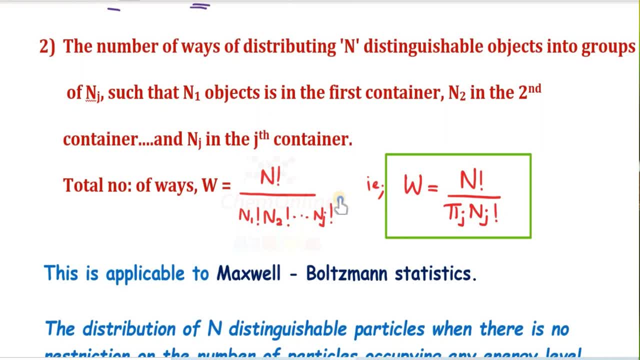 then the strengths of N- y. You just need to go ahead and put units of N and okay, you can go ahead and click the suit button. So, in other words, the levels of니까 First group or first container buttons are getting this. where you are getting this complex, you are getting 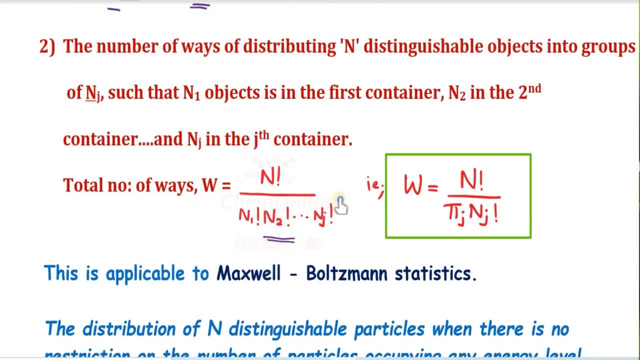 two, this simple WILL principles on the H into N2 factorial etc. up to NJ factorial. That is, W equals N factorial divided by the whole of NJ factorial, or we may say the product of NJ factorial. Now this is applicable to Maxwell-Boltzmann statistics. 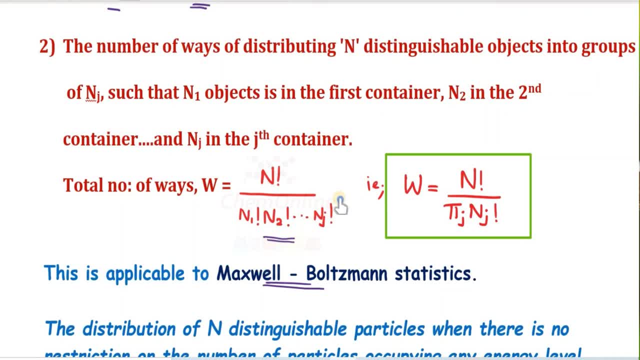 When we see Maxwell-Boltzmann statistics, the particles are distinguishable and any number of particles can occupy the energy level, same energy level. Similar is the situation here. We have N distinguishable objects and they can be arranged like N1 objects in the first. 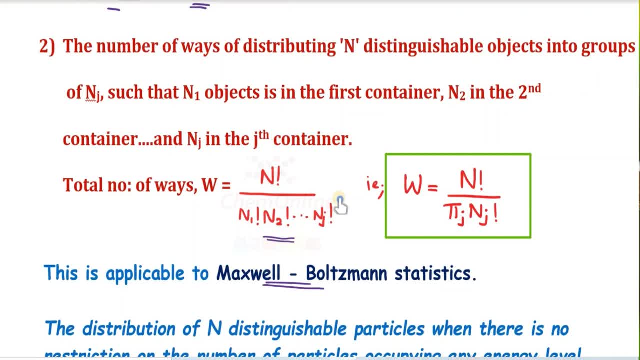 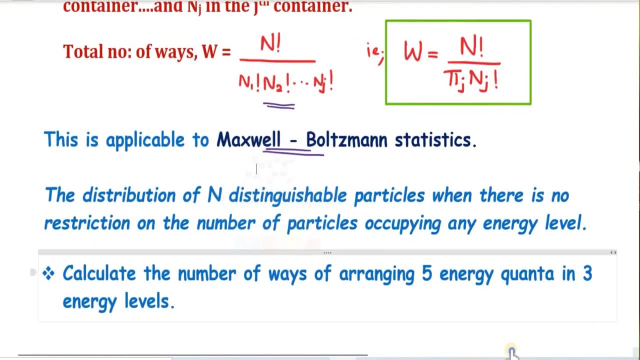 N2 objects in the second, etc. So the equation will be: W equals N factorial by the product of NJ factorial. So this is applicable to Maxwell-Boltzmann statistics, that is, the distribution of N distinguishable objects where there is no restriction on the number of particles occupying 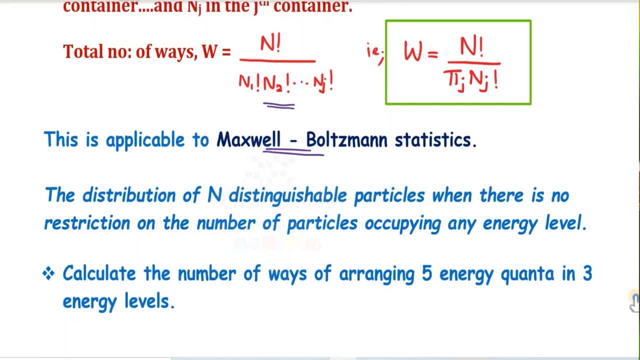 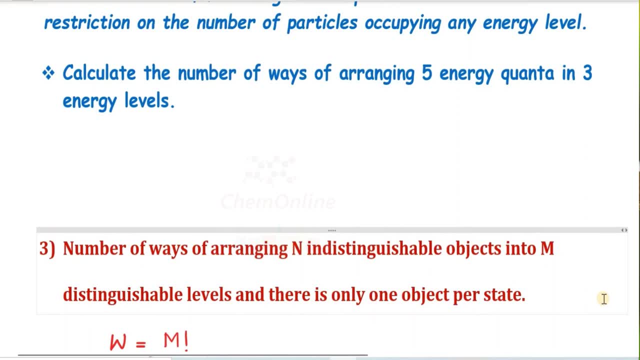 any energy. So we will see one example: Calculate the number of ways of arranging 5 energy quanta in 3 energy levels. We have 5 energy quanta. That means the number of particles is 5 and you have to arrange it in 3 energy levels. There is no restriction on the number of particles in each energy level. 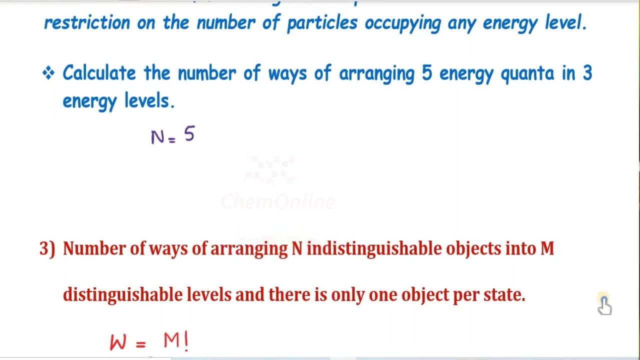 So we have N equals W equals N factorial. So this is applicable to Maxwell-Boltzmann statistics: W equals 5 and W equals N factorial divided by total of NJ factorial. So that is equal to 5 factorial divided by. we have 3 energy levels, So N1 factorial into N2, factorial into N3. 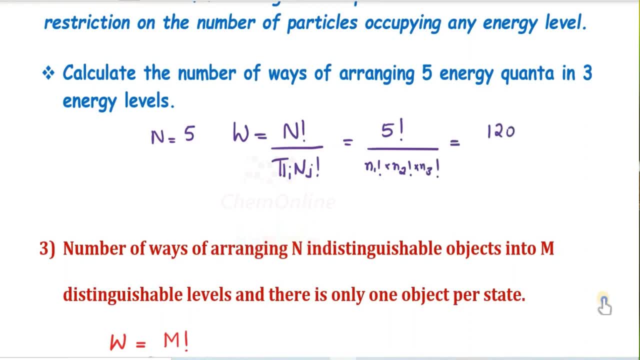 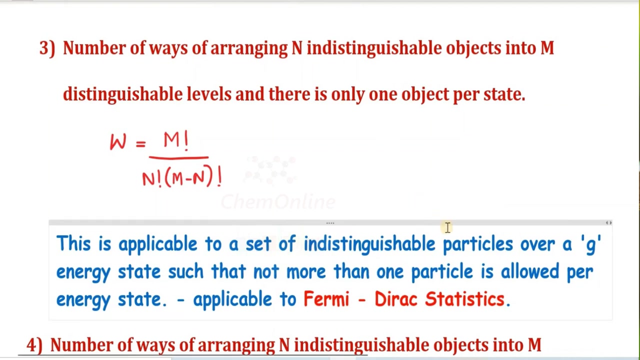 factorial. So that is equal to 120 divided by 2 into 6. So that is equal to 10.. So we have calculated the number of ways of arranging 5 energy quanta in 3 energy levels. The next is number of ways of arranging N indistinguishable objects into M distinguishable. 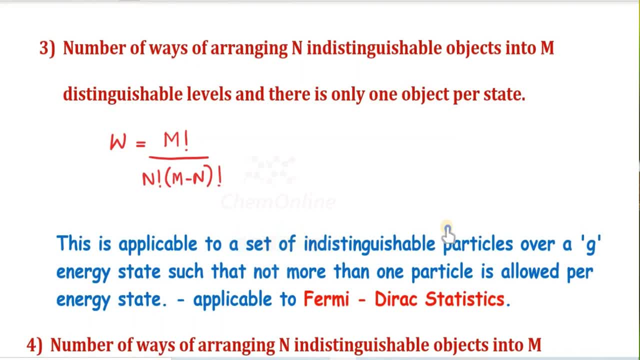 levels And there is only one object per energy state And the equation is given as: W equals M equals W equals N factorial into N2 factorial. So this is applicable to Maxwell-Boltzmann statistics: W equals M factorial divided by N factorial into M minus N factorial, And this is applicable. 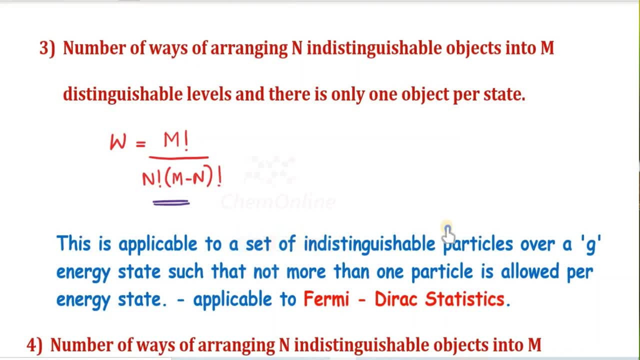 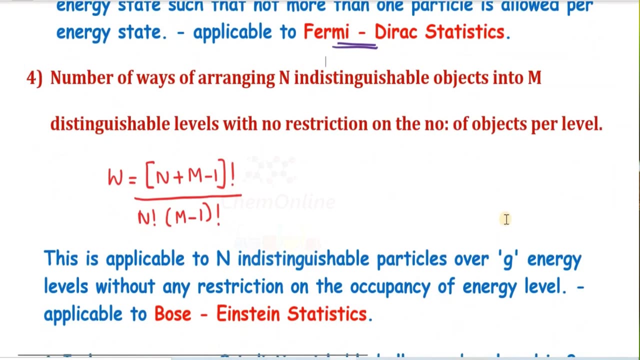 to a set of indistinguishable particles over an energy state, such that there is only one particle or one object in each energy state, And this is applicable to Fermi-Dirac statistics. Now, next is number of ways of arranging N indistinguishable objects. 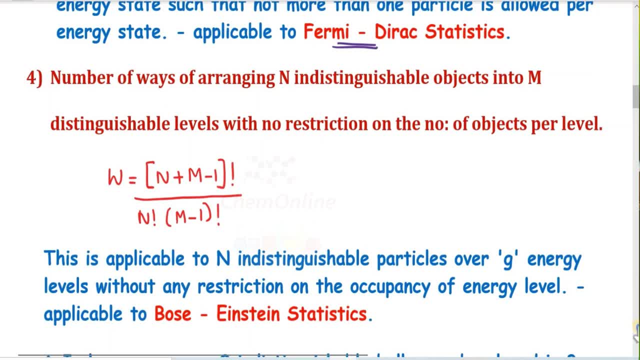 into M distinguishable levels with no restriction on the number of objects per level. So again, here also the particles are indistinguishable, but no restriction on the number of objects. So W equals N plus M minus 1 the whole factorial divided by N factorial into M minus 1, the whole. 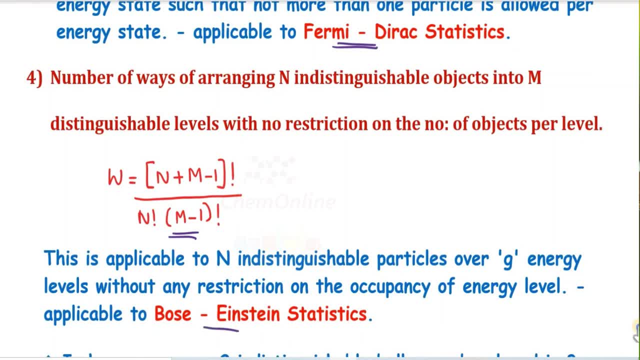 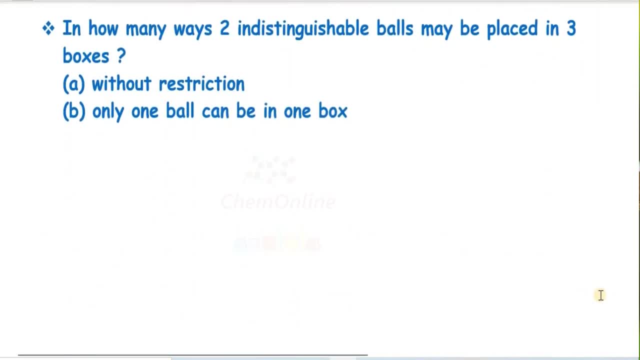 factorial, And this is applicable to Bose-Einstein statistics. Let us look at another example: In how many ways two indistinguishable balls may be placed in three boxes. A- without restriction. B- only one ball can be in one box. So you have two indistinguishable balls And how it can be placed in three boxes. 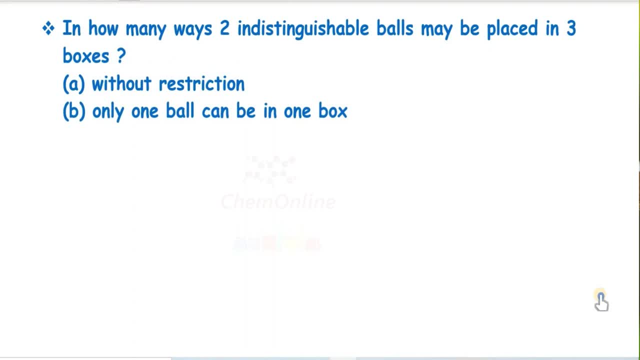 So first case we will see without any restriction. So then the equation is: W equals N plus M minus 1 the whole factorial divided by N factorial into M minus 1 the whole factorial. And this is applicable to Fermi-Dirac statistics. And this is applicable to Fermi-Dirac statistics. So then the equation is: W equals N plus M minus 1 the whole factorial divided by N factorial into M minus 1 the whole factorial, And this is applicable to Fermi-Dirac statistics. And this is applicable to Fermi-Dirac statistics. 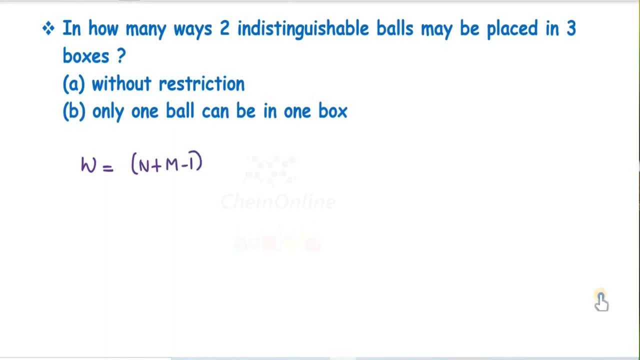 So then the equation is: W equals N plus M minus 1. the whole factorial divided by N factorial into M minus 1. the whole factorial. N is 2 plus M is 3 minus 1. the whole factorial divided by 2 factorial into M minus 1: the whole factorial. 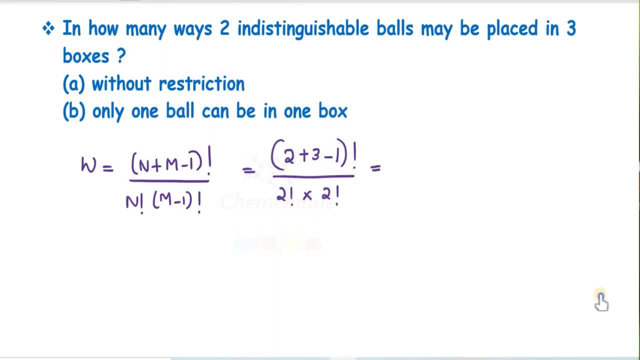 That is again 2 factorial, So that is equal to 4 factorial by 2. So that is equal to 4. factorial means 4 into 3, into 2, into 1, divided by 4. So that is equal to 6.. 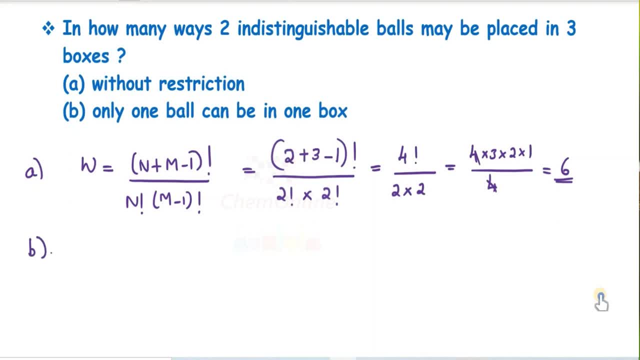 Now we will move on to B. Only one ball can be in one box. So we saw the equation: W equals M factorial divided by N factorial into M minus N. the whole factorial, So that is equal to M, is 3.. So 3 factorial divided by 2 factorial into 3 minus 2, 1 factorial. 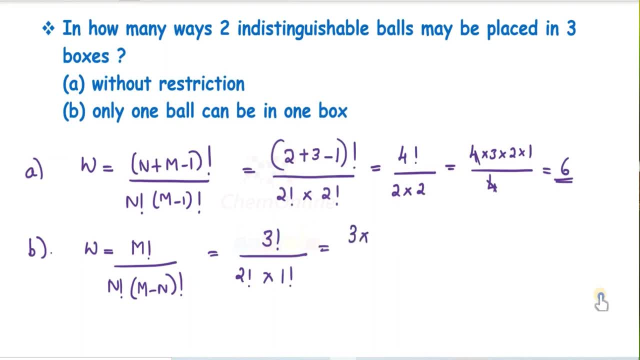 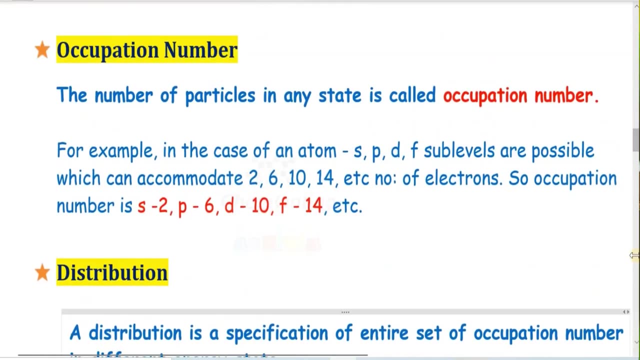 So that is equal to 3. factorial is 3 into 2 into 1. divided by 2, factorial is 2 into 1, 2. So that is equal to 3.. Now we will see about some basic terms that we use. 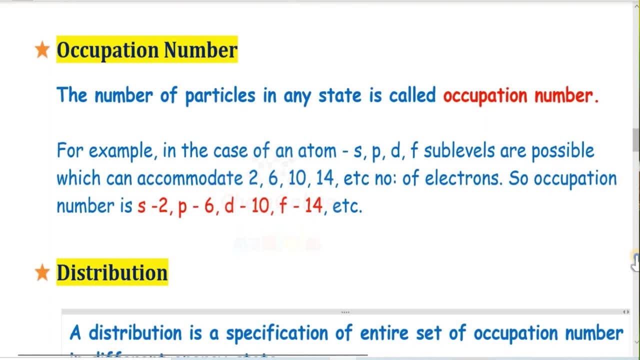 In statistical thermodynamics. The first one is occupation number. The number of particles in any state is called the occupation number. The number of particles in any state is called the occupation number. To be clear, we will consider the case of an atom. 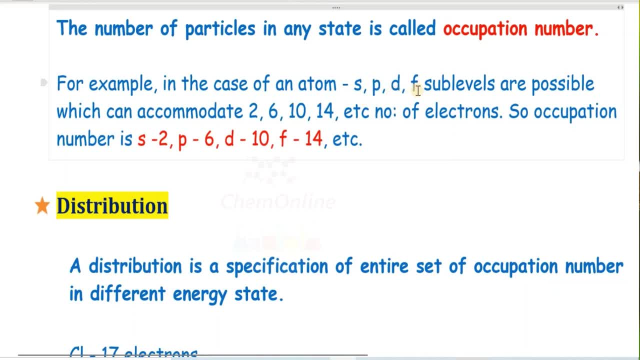 In the case of an atom we have different sub-levels, like S, P, D, F etc. And each sub-level we know that They can accommodate. for S can accommodate 2 electrons, for P 6 electrons and D 10 electrons. for F 14 electrons etc. 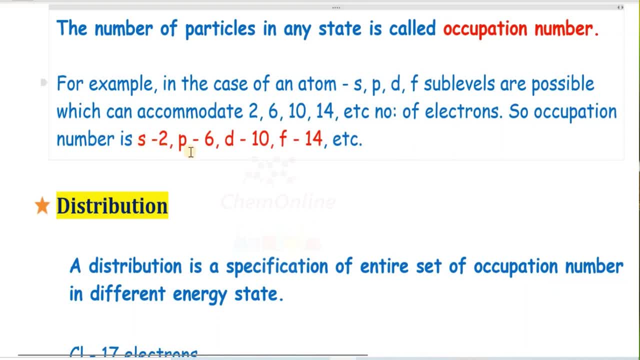 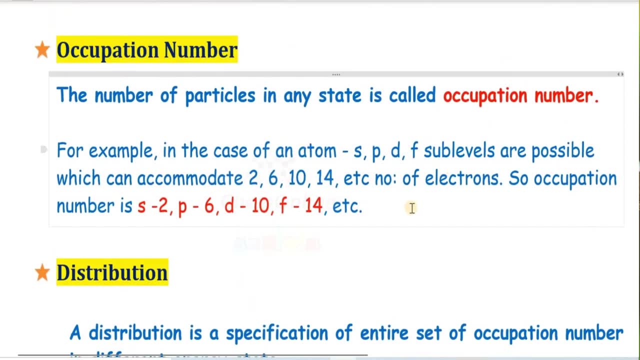 So we can say that the occupation number for S is 2,, P is 6,, D is 10,, F 14, etc. So this is what is meant by occupation number, the number of particles in any state. The next is distribution. 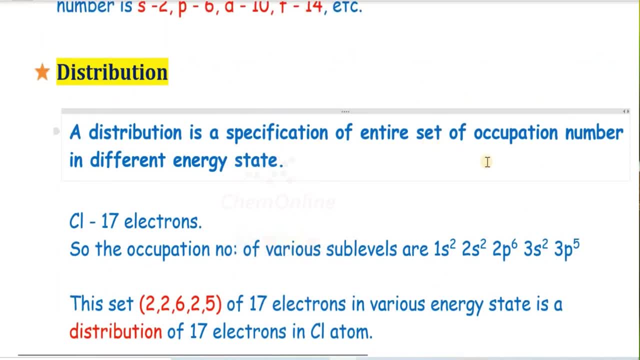 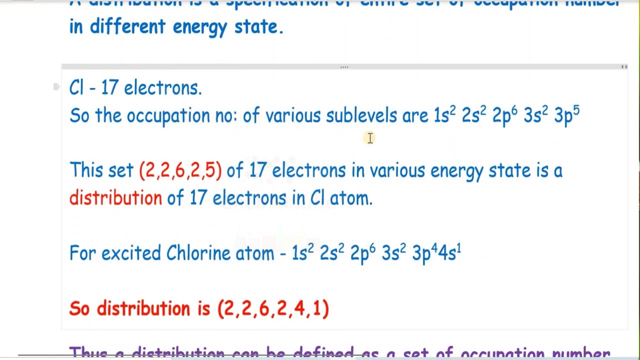 A distribution is a specification of entire set Of occupation number in different energy state. For example, consider chlorine. Chlorine has 17 electrons. So we can represent occupation number of various sub-levels By writing the electronic configuration, That is, 1S2, 2S2, 2P6, 3S2, 3P5.. 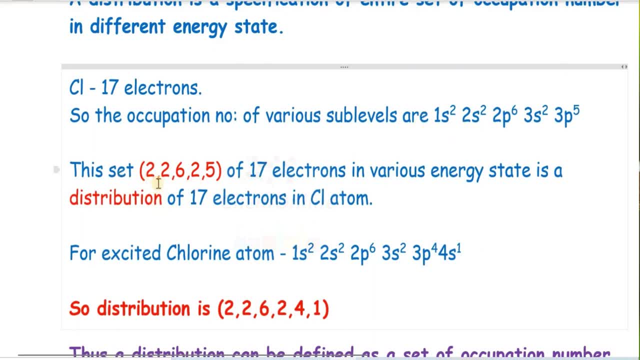 So we can say that this set, that is, 2,, 2,, 6,, 2,, 5.. Which constitute total of 17 electrons In various energy states There is a distribution of 17 electrons in chlorine atom. This is one way of distribution of 17 electrons in chlorine atom. 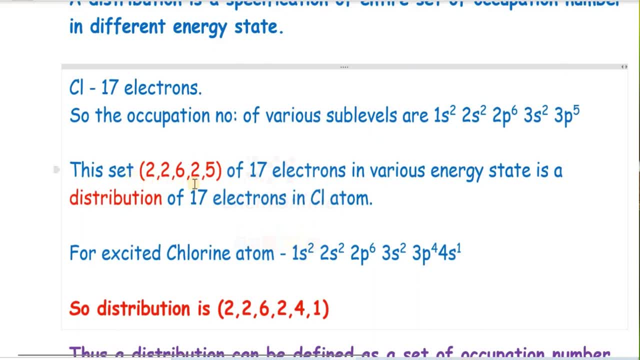 Now, if you consider the chlorine atom in the excited state, Then the configuration will be 1S2, 2S2, 2P6, 3S2, 3P4, 4S1.. So one electron from the 3P is excited to 4S. 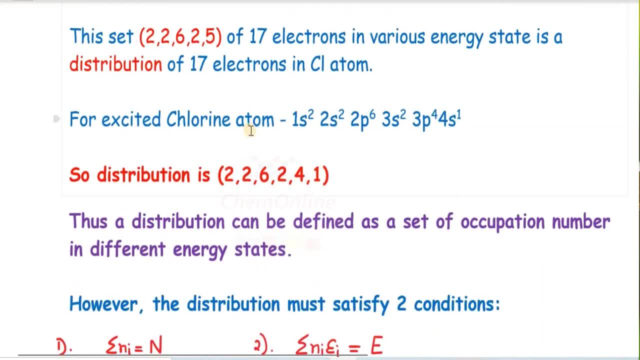 Now, if you consider the chlorine atom in the excited state, Then the configuration will be 1S2, 2S2, 2P6, 3S2, 3P4, 4S1.. Now the distribution will be 2, 2, 6, 2, 4, 1. okay. 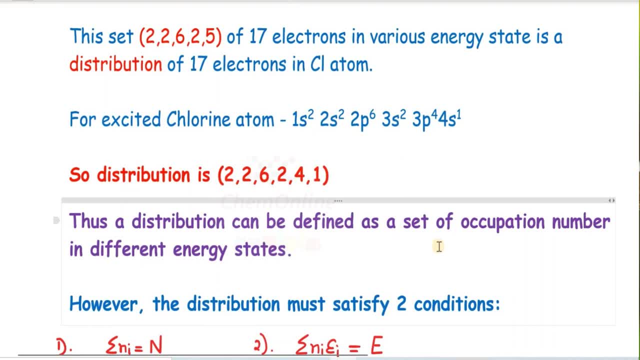 So we can say that a distribution is defined as a set of occupation number In different energy states. Another important element of distribution are its Hall particles. So he did not know any about that. He can only look at energy state. Occupation number is the number of particles in each energy state. 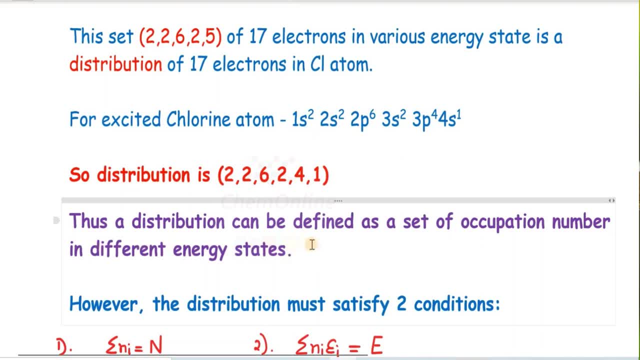 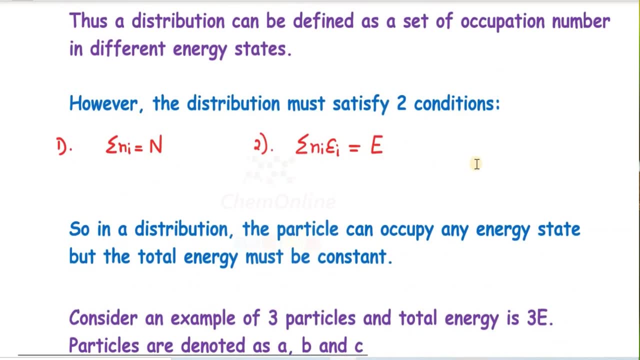 and a distribution is a set of occupation number in different energy states. But a distribution must satisfy two conditions: Summation Ni equals capital N, That is, the total number of particles should be a constant, that is N, capital N. And also summation Ni, epsilon I equal to capital E. 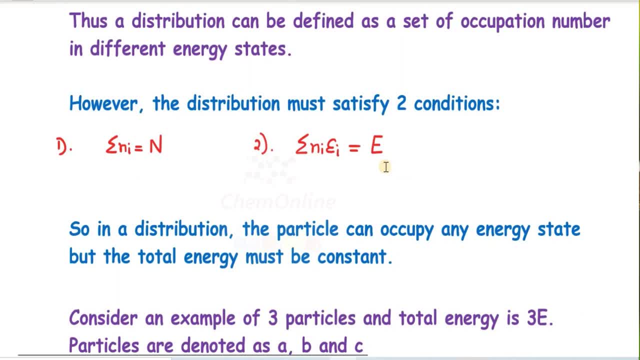 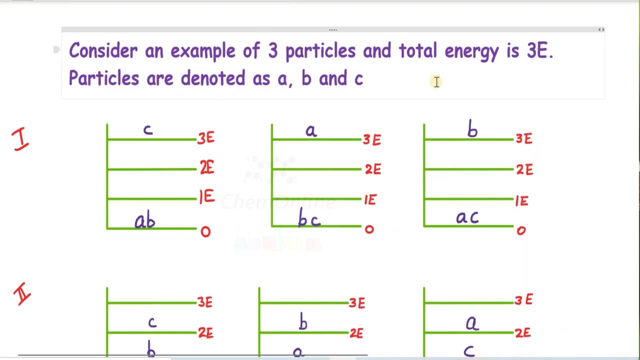 The total energy must also be a constant. So distribution must satisfy two conditions: Summation Ni equals capital N and summation Ni epsilon I is equal to capital E. So we are considering an example of three particles, and the total energy is 3E, which is a constant. 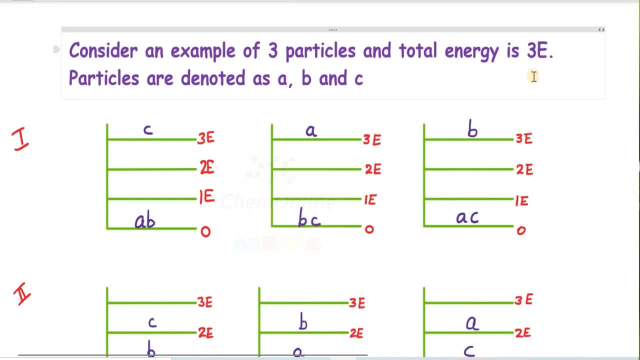 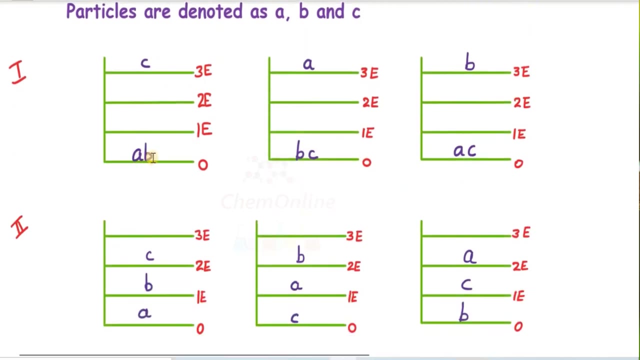 So we have three particles. The total energy must be a constant 3E. The particles are denoted as A, B, C, etc. We are going to see how these particles can be arranged in the energy levels, So either the two particles, A and B, in the zeroth level and the remaining one, C, in the third level, having energy 3E. 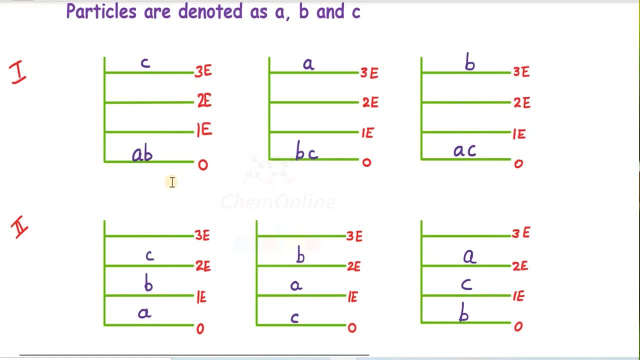 So the total energy will be 3.. Now another arrangement is here Here: B and C in 0,, whereas A in 3E, So again the total energy will be 3.. And the last one is: A and C in the zeroth level and B in 3E. 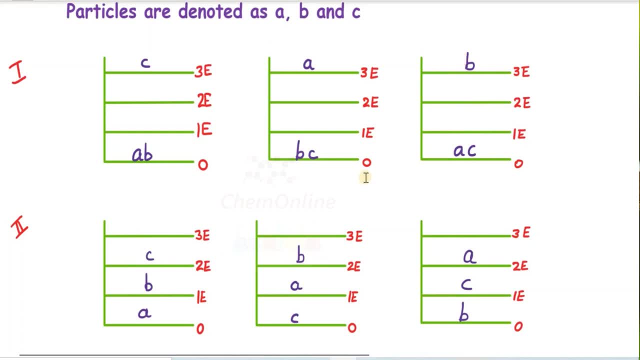 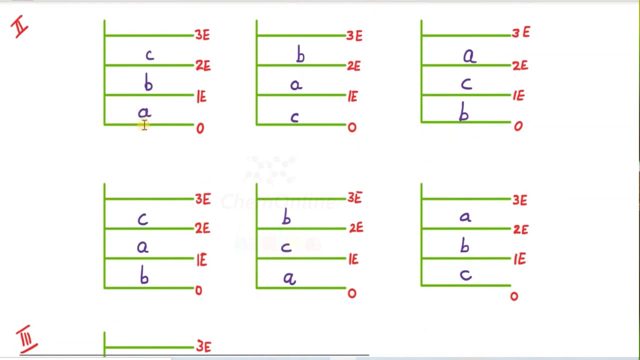 So here also the total energy will be 3.. So this is a group of arrangement. Now, which way to arrange? The total energy is 3E. So the second type: one particle having energy 0, the second one having energy 1E and the third one having energy 2E. 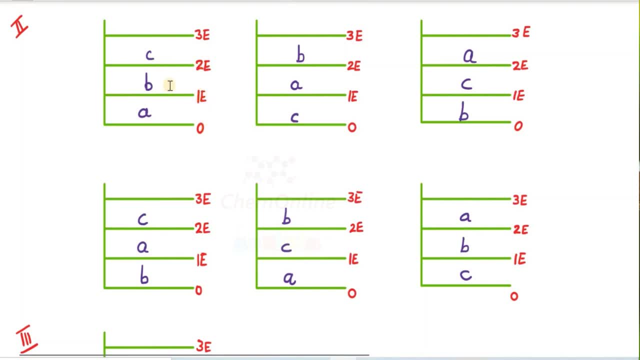 So that the total energy will be 0 plus 1 plus 2, 3E. Similarly, you can arrange it as CAB, BCA, BAC, ACB, CBA. Okay, In this way, you can arrange it as 6.. 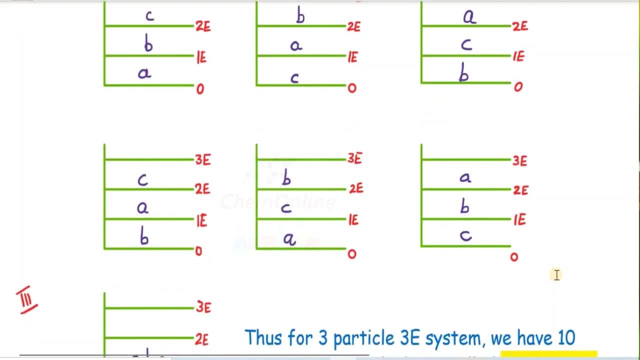 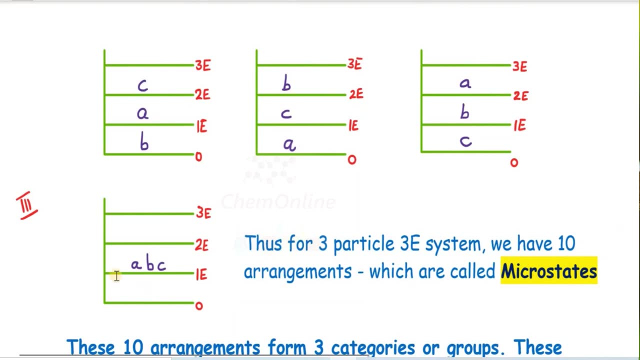 This is the different way it is arranged here. Now there is one more way in which you can arrange the particles so that the total energy will be 3E, Where the new particles in you keep A, B and C is the first energy level. 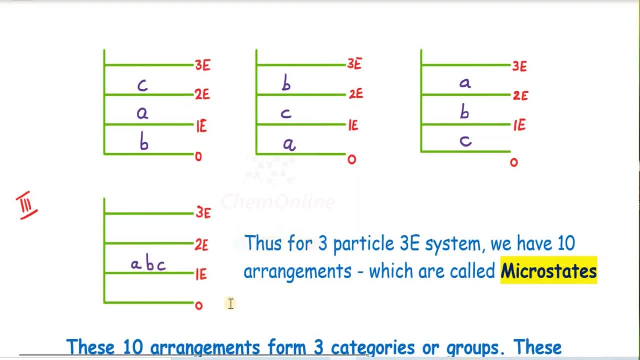 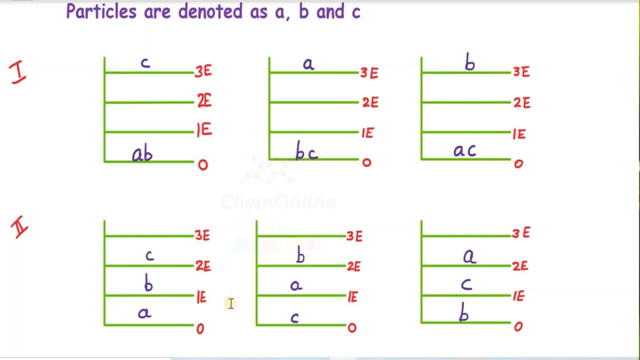 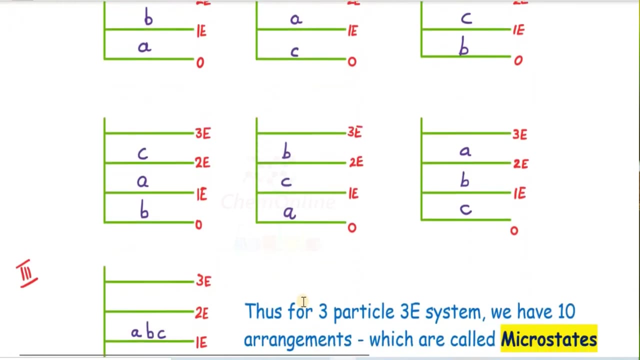 So that the total in energy will be 3E. You have three particles, marked AB and C, And you have arranged the particles in different energy levels. the total energy is a constant, which is 3.. Okay, So you have these different kinds of arrangement. 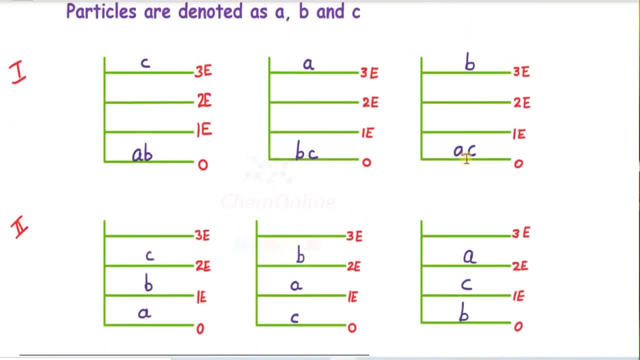 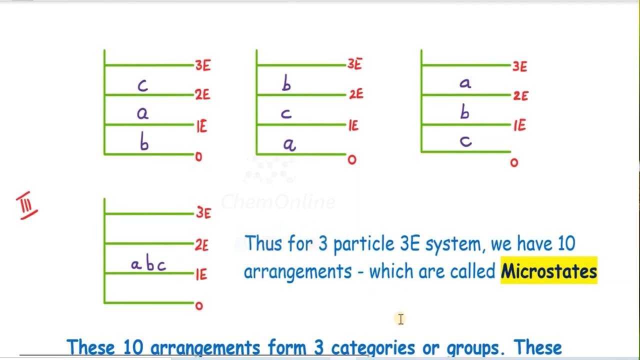 So, total, you have 10 arrangements, Okay, So the first one is 3.. The second one is 6.. So 3 plus 6,, 9 plus 1, 10.. So we have 10 arrangements, and these 10 arrangements are called. 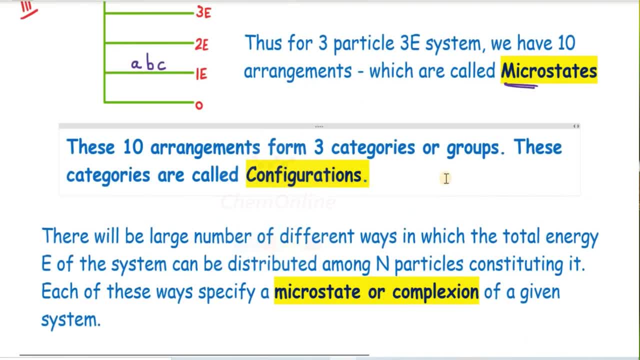 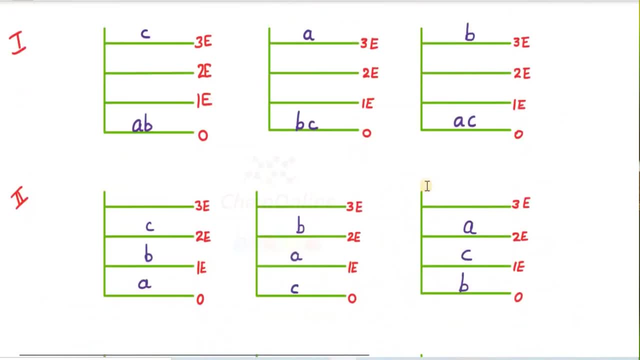 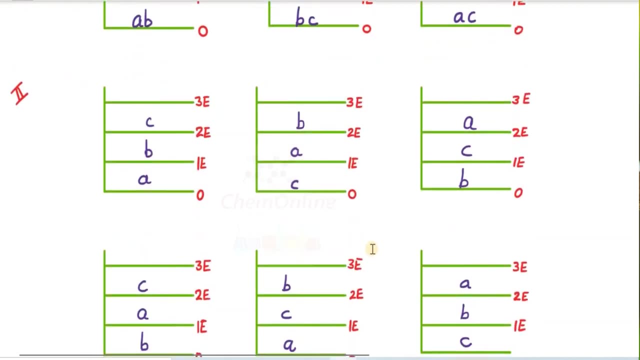 microstates, And these 10 arrangements form 3 categories or groups, and these categories are called configurations. Okay, In the first configuration you have 3 microstates. In the second configuration you have 6 microstates. and the third configuration. 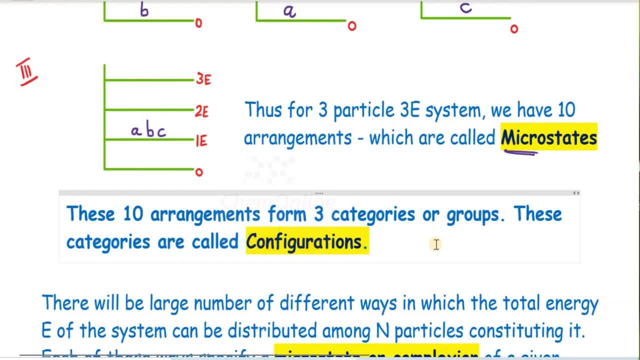 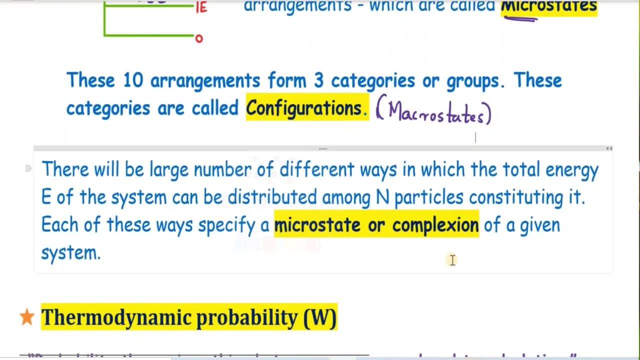 you have 1 microstate, Okay, And this configuration is also known as macrostates. So under each configuration or macrostate you will have different microstates. So here you can see that there are a large number of ways in which the total energy of the system 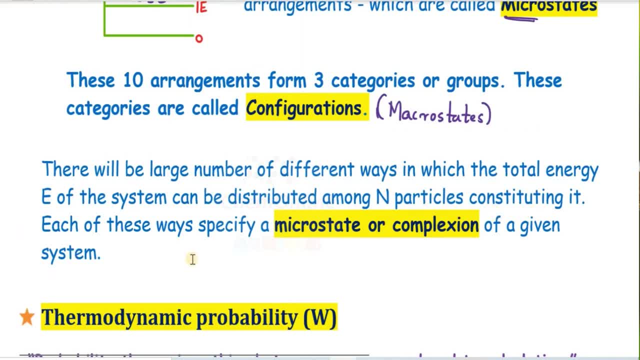 can be distributed among n particles, And each of these ways specify a microstate or complexion. Another name for microstate is complexion of the given system. Now next is thermo energy. So thermo energy is a complexion of the given system. So thermo energy is a complexion. 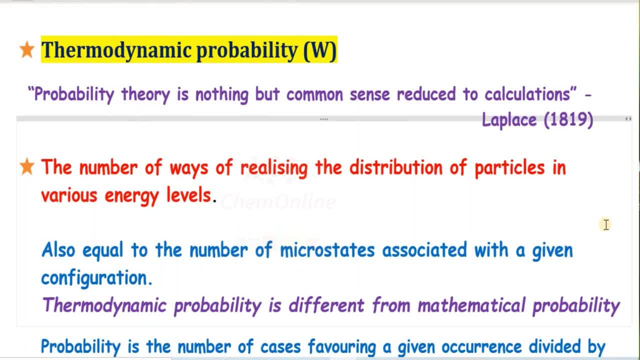 of the given system. Now, next is thermo. energy is a complexion of the given system. So thermo dynamic probability, Statistical thermodynamics, is a quantity which is most important when you learn it. All right, So let us see what is Thermodynamic probability. 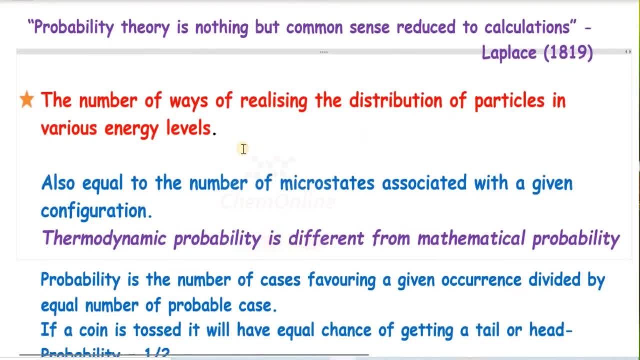 The number of ways of realizing the distribution of particles in various energy levels is thermodynamic probability. How can particles be distributed at different energy levels? So the number of ways of realizing the distribution of particles in various energy levels is thermodynamic probability. Thermodynamic probability is also equal to the number of microstates associated with a given. 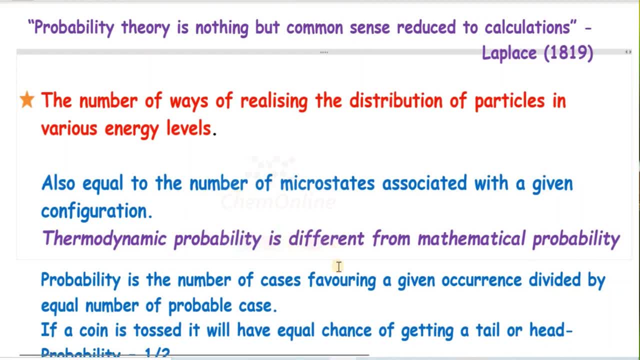 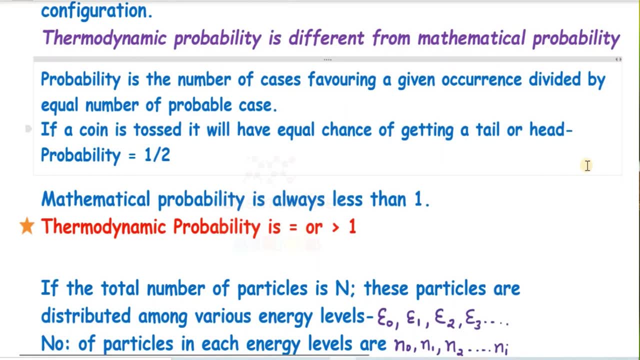 configuration. Thermodynamic probability is different from mathematical probability, So let us see what is mathematical probability. If we toss a coin, either you will get tail or you will get head. There is an equal chance of getting a tail or head. So we say that the 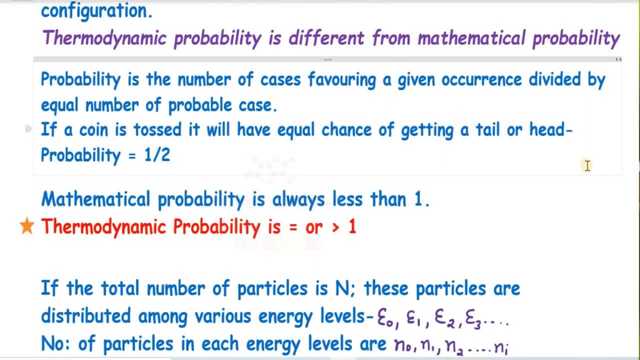 probability is 1 by 2.. So there are two possible chances. Out of that two, only one is possible. So the probability is 1 by 2.. So mathematical probability is the number of cases favoring a given occurrence divided by equal number of probable case. So mathematical probability, 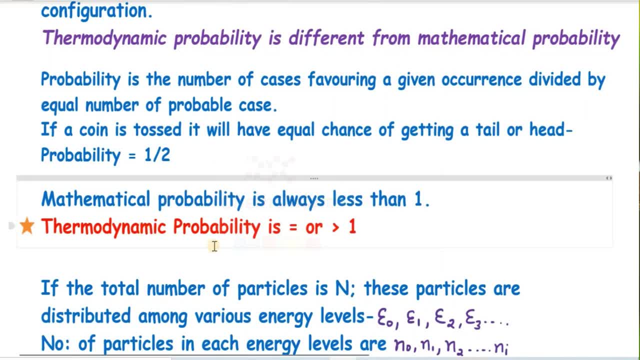 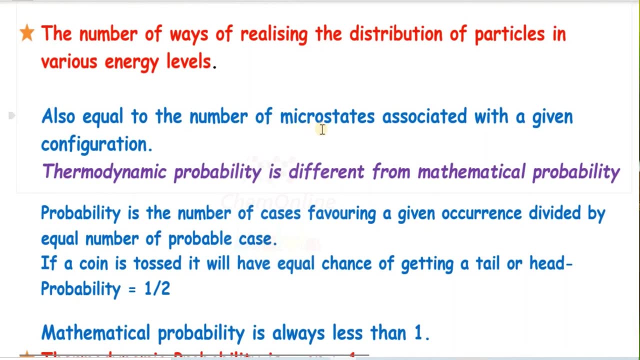 is always less than 1.. But thermodynamic probability is equal to or greater than 1.. Actually, it is a number between 1 and infinity, whereas mathematical probability is less than 1.. And thermodynamic probability is also equal to the number of microstates associated with a configuration: The total. 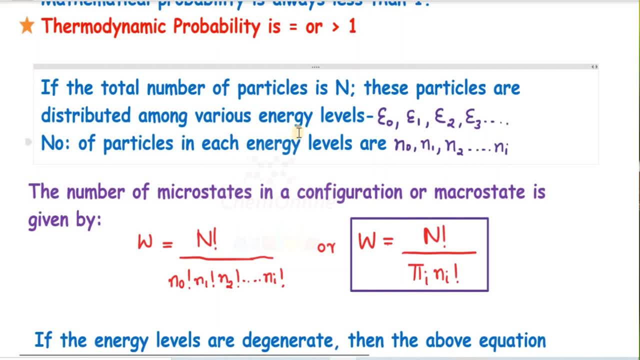 number of particles is n, and these particles are distributed among various energy levels, like epsilon 0, epsilon 1, epsilon 2, etc. And the number of particles in each energy levels is n0,, n1,, n2, etc. to n9. 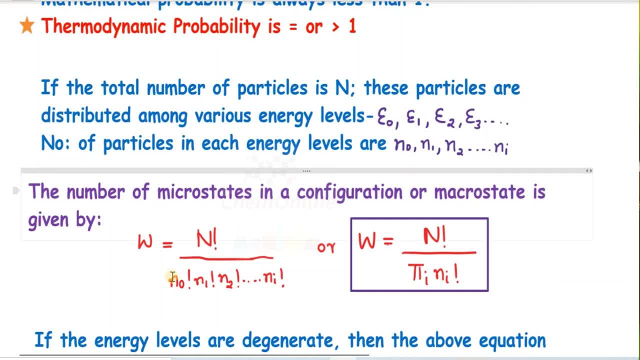 And the number of microstates in a configuration is given by w equals, or we can call it thermodynamic probability. w equals- thermodynamic probability is always represented by w. w equals, n factorial, by n0, factorial n1, factorial n2, etc. to n. Or you can write n factorial. 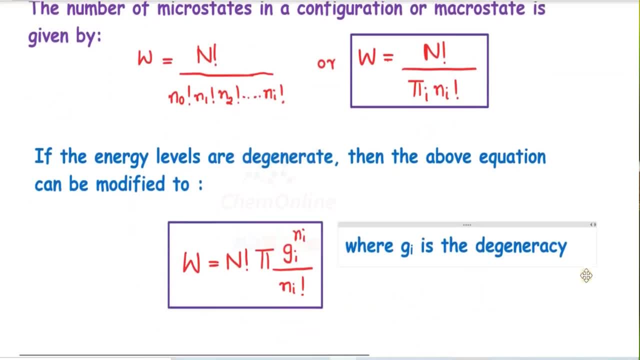 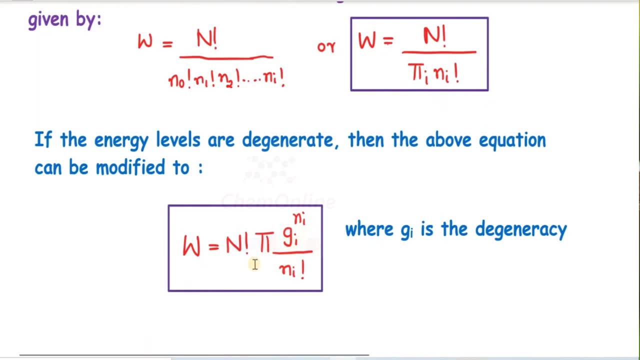 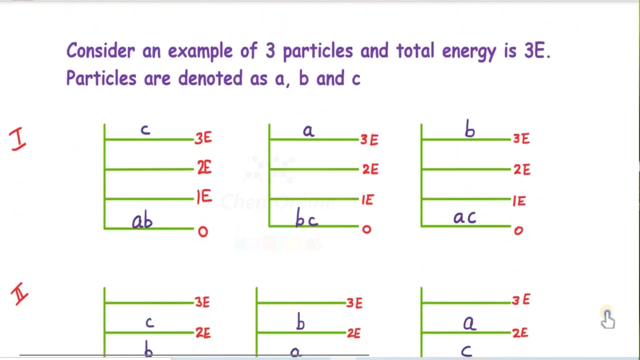 by product incorrectness of ni factorial. And if the energy levels are degenerate, then this equation can be modified to w equals n factorial into product of gi raised to ni by ni factorial, where gi is the degeneracy of the energy level. Now let us look at this example: three particle, three energy. 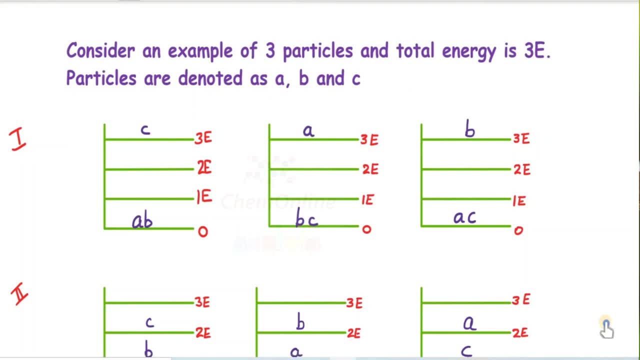 In the first case, how can we calculate the probability of this? So w1, first arrangement. w1 is equal to total energy factorial divided by two factorial into one factorial, That is, two particles in one energy level and one particle in another energy level, That is, three factorial. by 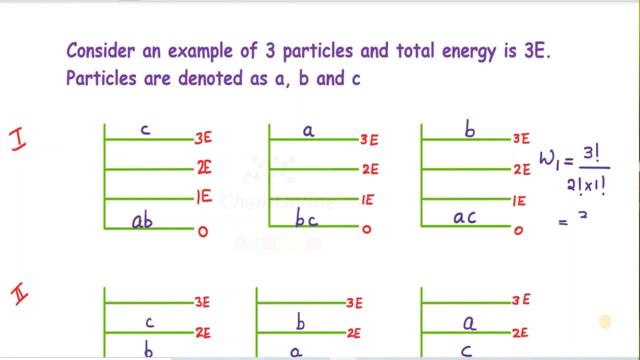 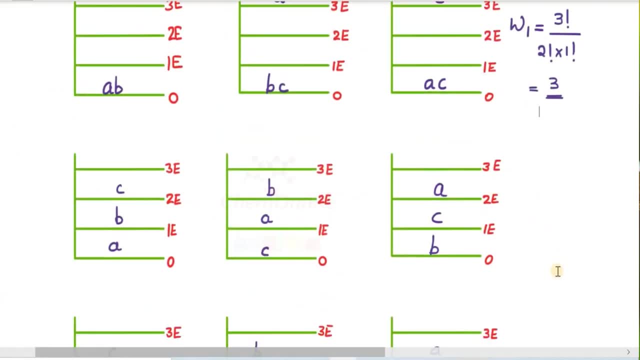 two factorial into one factorial. So that is equal to three. That means the number of microstates is three And that is what we represent as three microstates. Now we consider the second configuration. Second configuration: you have six arrangements. 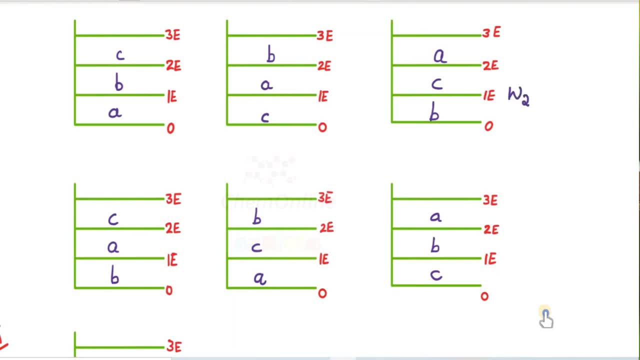 So let us see the thermodynamic probability That is. w2 equals three factorial divided by one factorial into one factorial, into one factorial. That is equal to six. So we have six kinds of arrangement, or we say that there are six number of microstates. 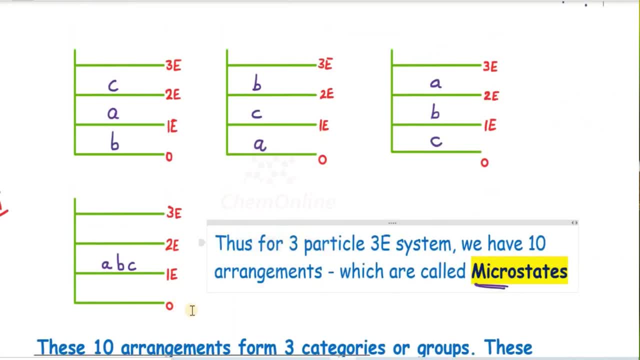 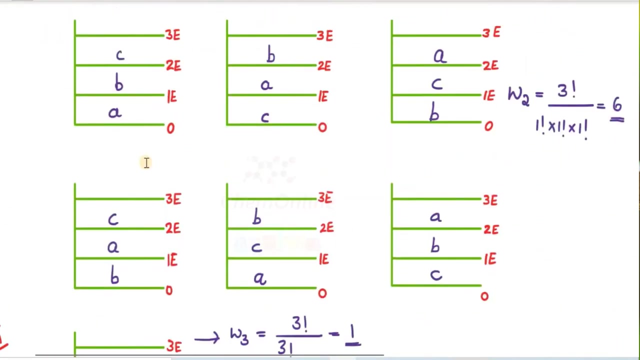 And the third one. there is only one type and the probability can be calculated as: w3 equals three factorial by three factorial, So that is equal to one. Here only one microstate. We move on the configuration in compare aimball. The second configuration has the maximum number. 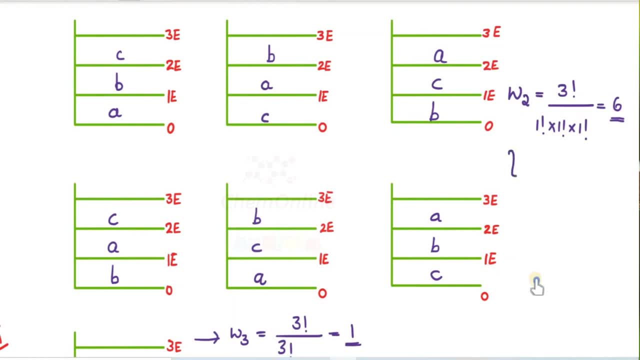 of microstates. So we can see that the number of microstates is three. So we can see that the number of microstates is three. So we can see that the number of microstates is three. So we can say that this configuration is the most probable configuration, since it has the maximum number. 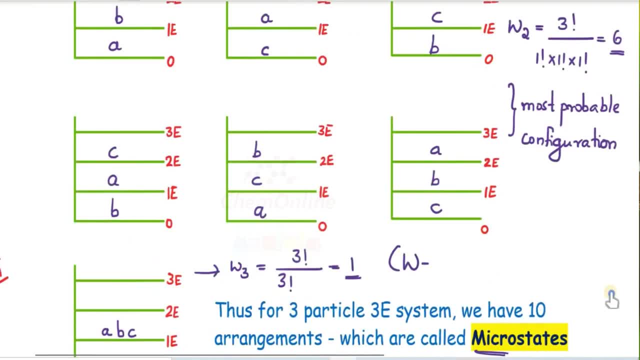 of microstates, The total thermodynamic property w is equal to the W1 plus W2 plus W3. So that is equal to three plus six plus one, which is equal to ten as the total probability, which is again equal to the total number of microstates. Sorting out part three of the affirmations. 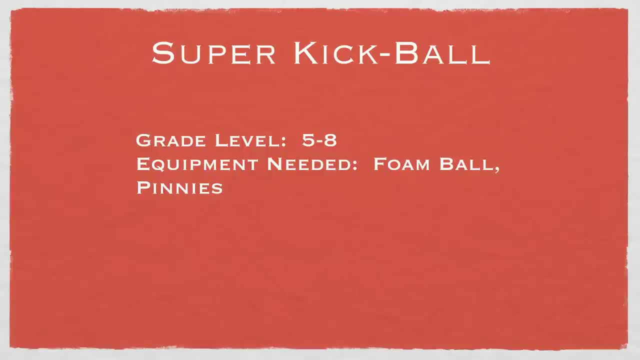 Hi, this game is called Super Kickball For grades 5 to 8, you're going to need a foam ball and pennies. So in this game you're going to use a basketball court, the lines from a court or, if you're outside, you can use cones or markers. 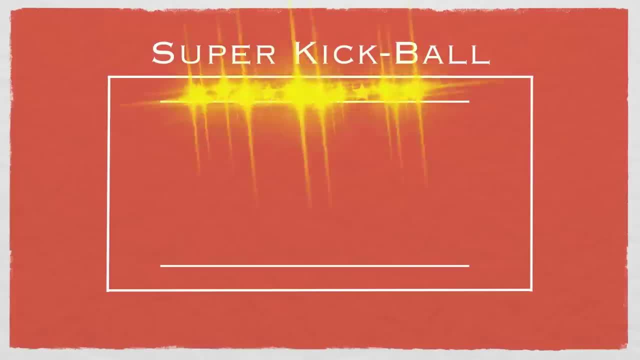 And you're actually going to use just the side lines from the court. You'll have one team, who will be the kicking team to start, that can wear pennies, and a fielding team as well in the playing area And, as a teacher, you'll start with the ball in the middle. 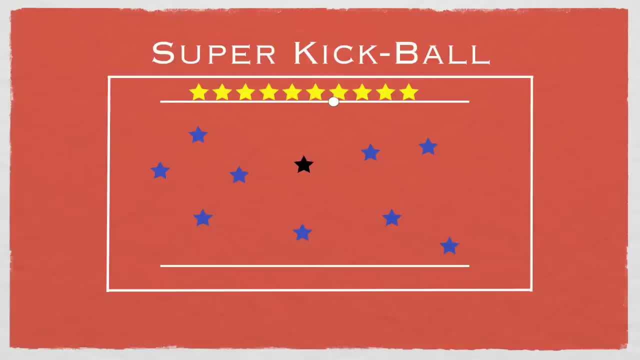 And when you start you'll roll. You'll choose a student to roll the ball to and that student will kick it. Now, what happens once the kick has been made is the whole team. so all of the yellow players will try and run to the other line on the other side and then back again.